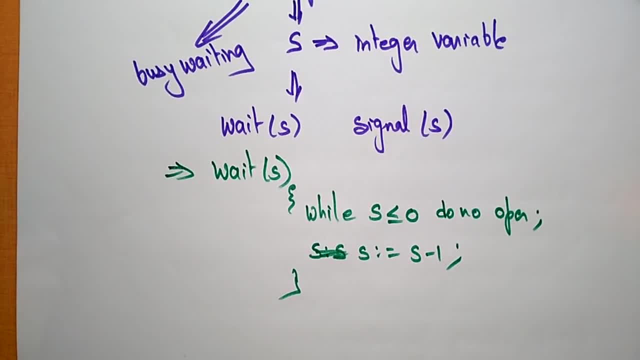 So this is the code for the weight. And next, coming to this signal, Next atomic operation is signal, which is used by the semaphors. variable Signal s Signal s indicates: s is equal to s plus 1.. So here weight is doing the operation as a decrement operation. 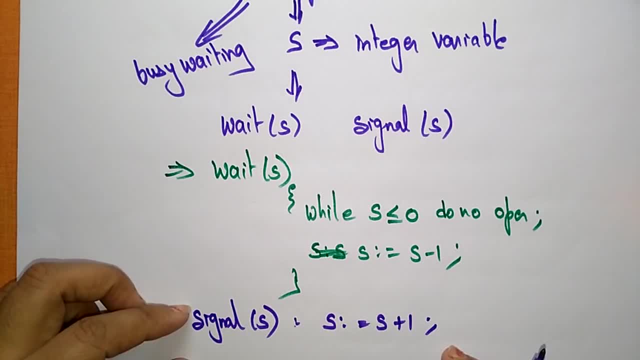 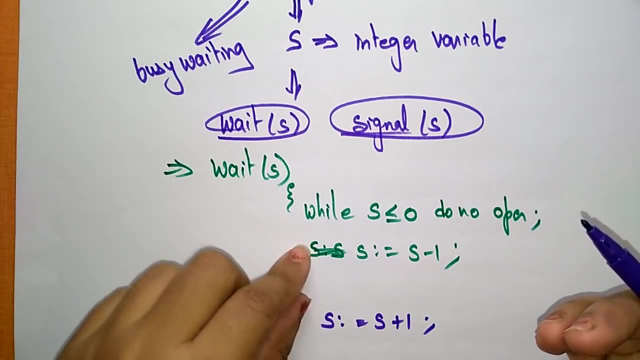 And the signal is Using the operation as a increment operation. So why this semaphors is using these two atomic operations, weight and signal. Okay, So we know that whenever this while condition is satisfied, It will execute the program. Okay, Here there is no program. 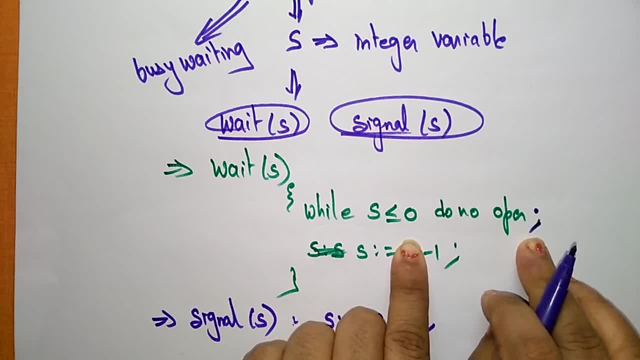 Why there is no program? Because it is ended with semicolon, While s less than or equal to 0. There is S less than or equal to 0. So this is the condition. So whenever the condition is satisfied, It doesn't do any operation. 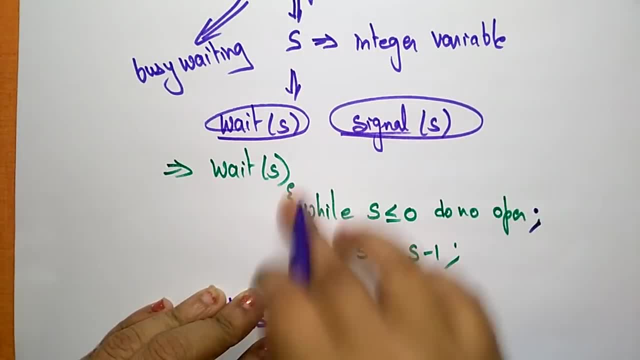 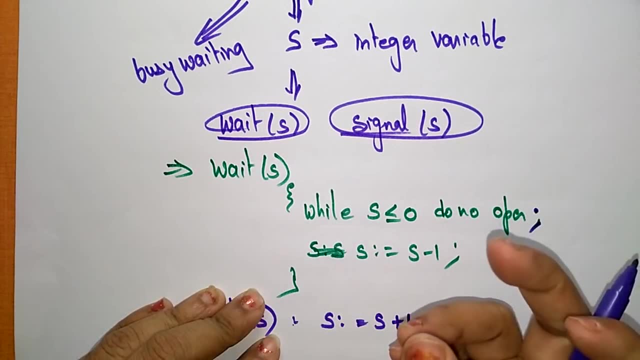 So it is continually rotating Means. it is in a loop condition only. So whenever this condition is satisfied It has to be in a busy waiting. So we have to take care that This condition doesn't satisfied. Then only the process will be executed without busy waiting. 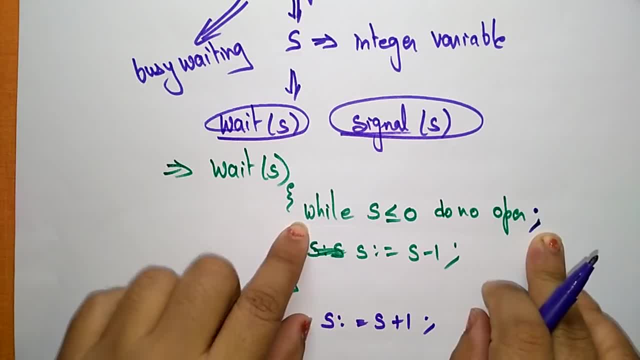 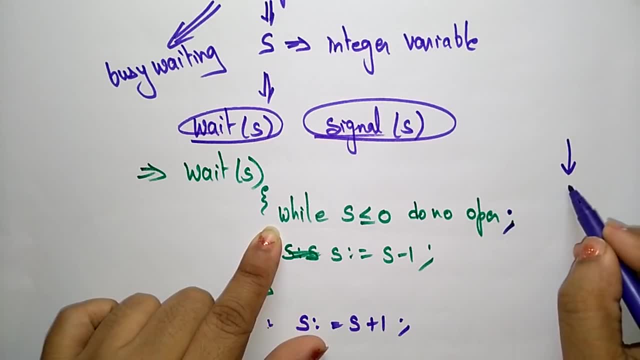 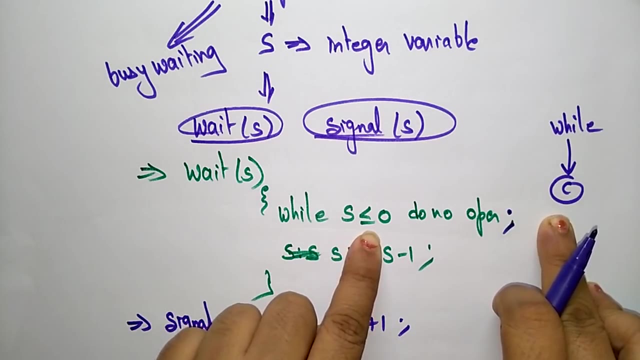 So that's why we have make it as a semicolon. Semicolon means this statement will be Ended. So we know that the while condition, So generally the while means the. whenever the while Check the condition first. it checks. the condition means s less than or equal to 0. 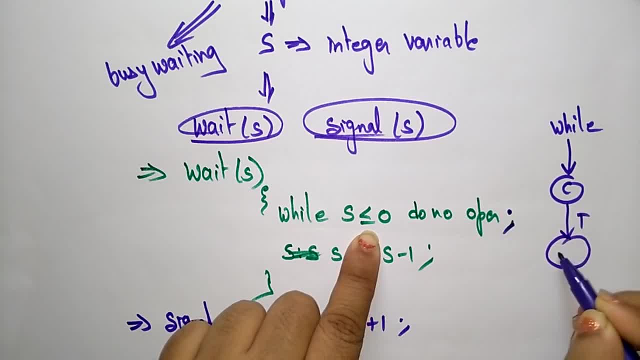 So whenever this condition is true, It enter into this statement. So it will execute until the statement is true, It checks the conditions and again it goes for the Another. checking the another condition, Again execute the statement. So if the condition is false, 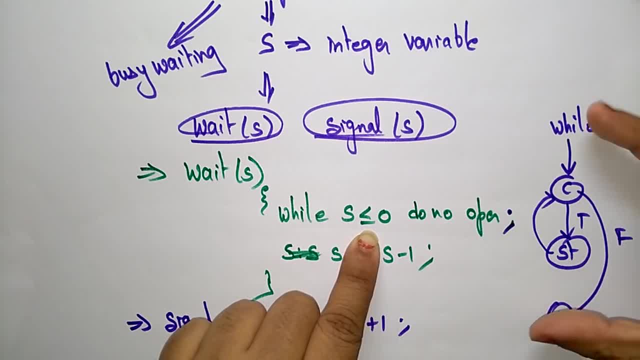 It exits from the loop. So this is actually the while operation. So here I'm saying while s less than or equal to 0.. Okay, do no operation means there is no code here. So whenever the condition is satisfied, there is no code to execute. 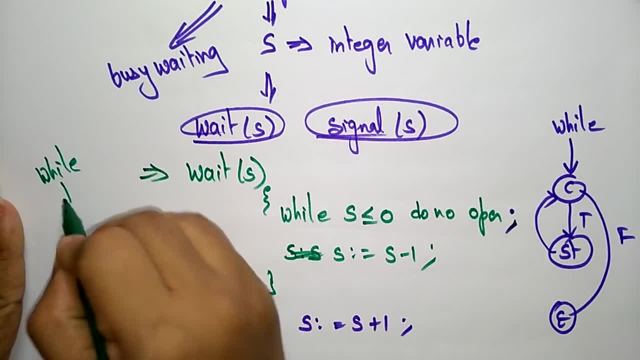 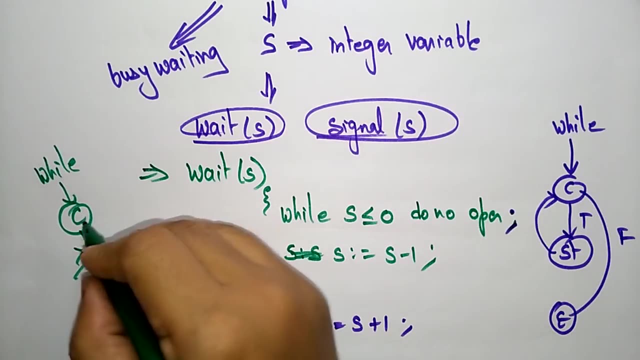 For this. So just here what it's a while Check the condition. So if the condition is satisfied it has to execute the statement. But there is no statement here. There is no statement, So compulsory it has to be exit, exit from the loop. 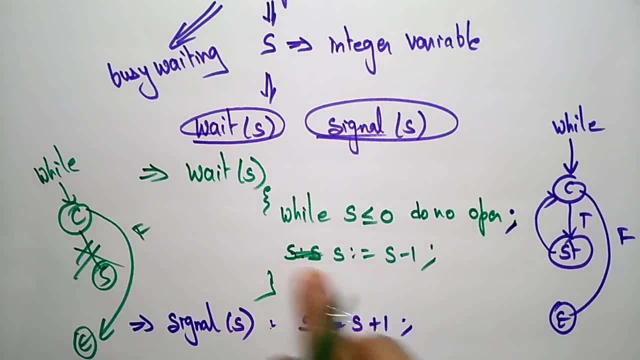 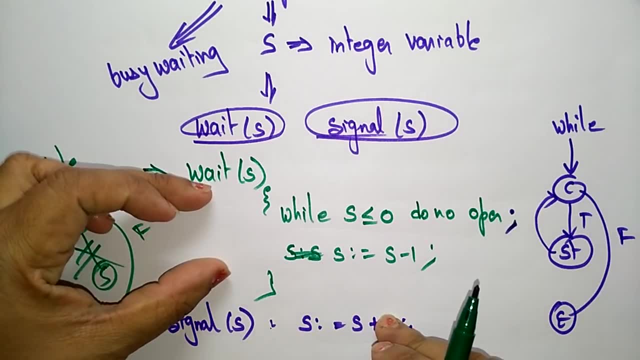 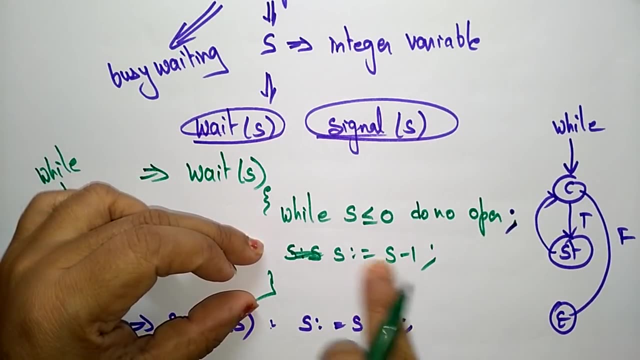 So that whenever the condition is satisfied, it exits from the loop and execute the next statement that is present in the code. So that's why we are using this wait operation. Okay, One process is executed, Executing without busy waiting. So why I'm decrementing this? s is equal to s plus 1 and I'm using the s is equal to s plus 1.. 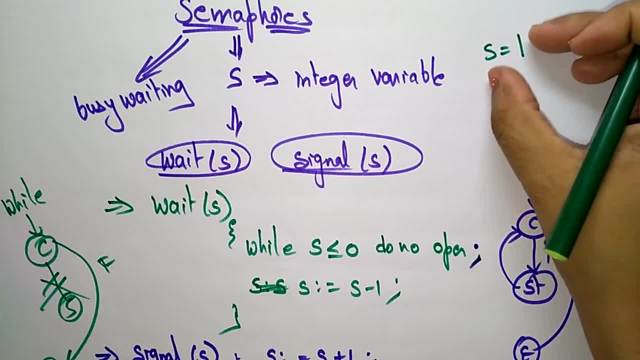 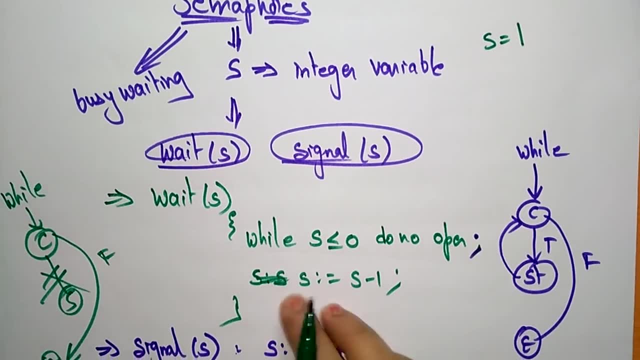 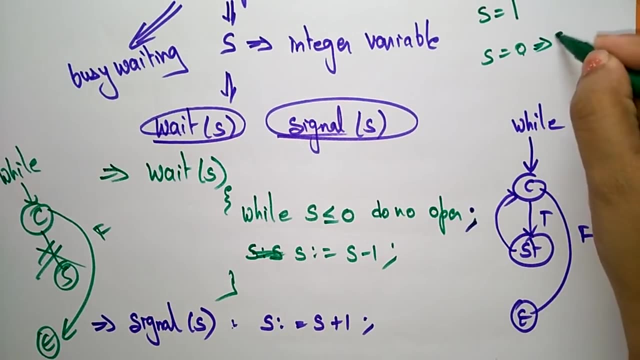 So whenever the sum of us value is 1, then only that process will enter into critical section. Other process will not enter into critical section. So after decrementing the value s becomes 0. So next another process means it saying that it is exit. 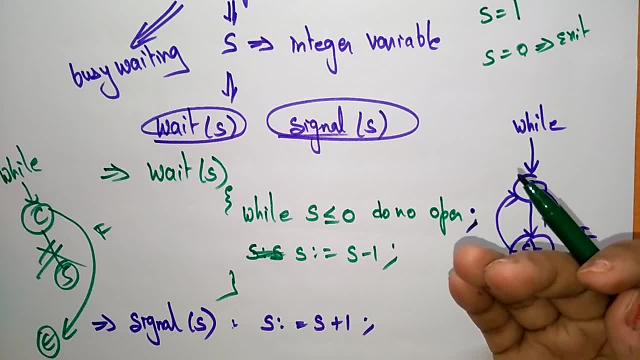 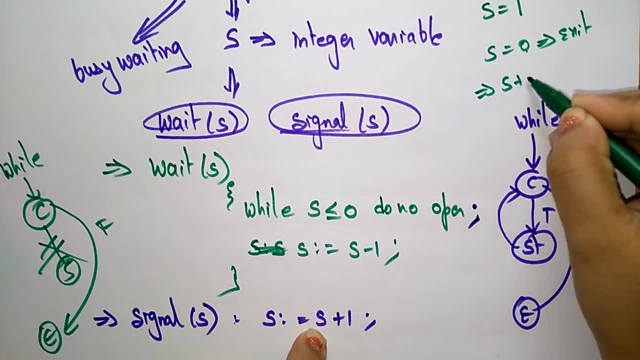 So if another process wants to execute again into the critical section. so that's why we are using signal operation, s is equal to s plus 1. here it is incrementing the s value as 1.. So then next process will enter into critical section. 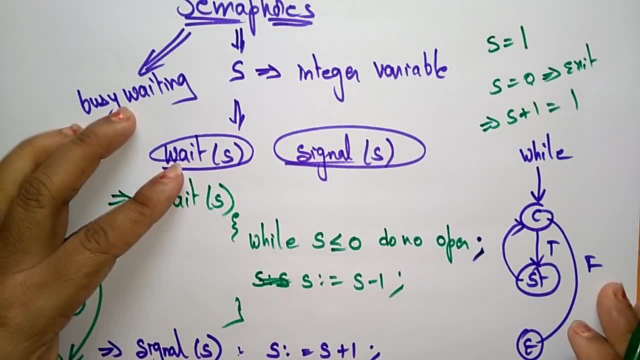 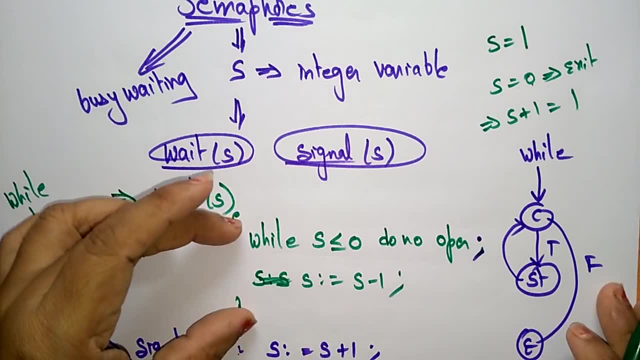 So that's the concept of sum of us, the sum of us here we are using that. it is a synchronization tool that does not require a busy waiting. so, without maintaining busy waiting, it is executing the process. So're executing the program By using to atomic cooperation. 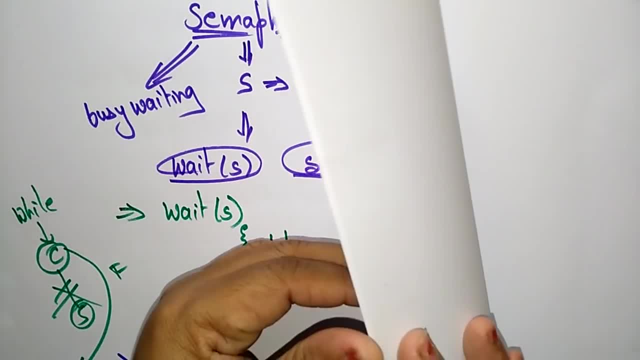 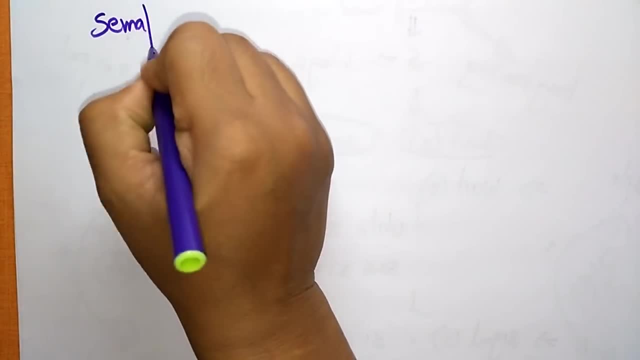 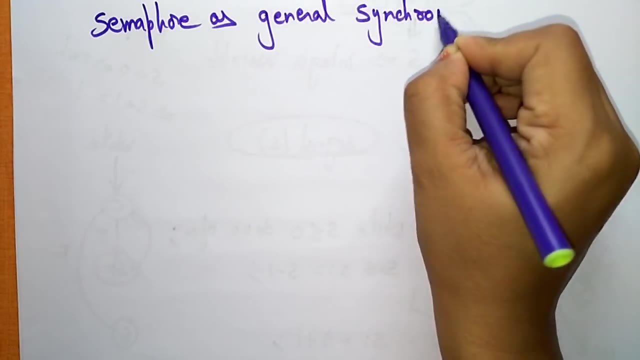 Wait and signal No liaseed the summer for some general synchronization. I said the sum of us as a general synchronization to let me explain that for some of bus as general synchronization Two That we use in the operating system How it is. 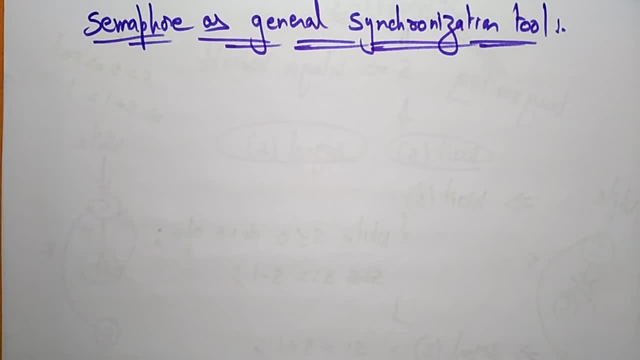 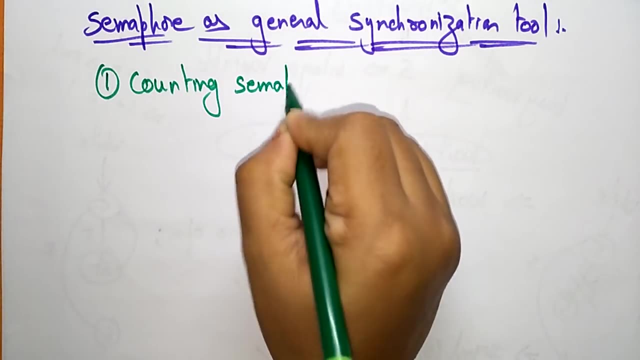 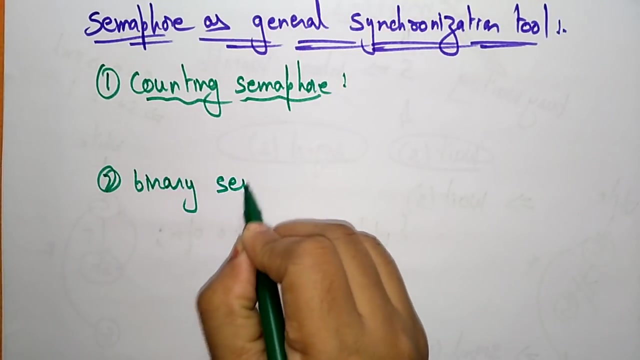 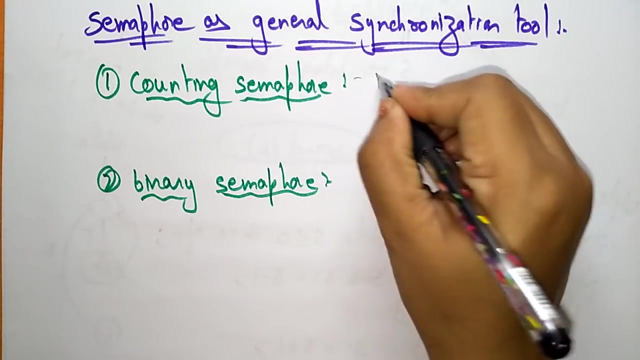 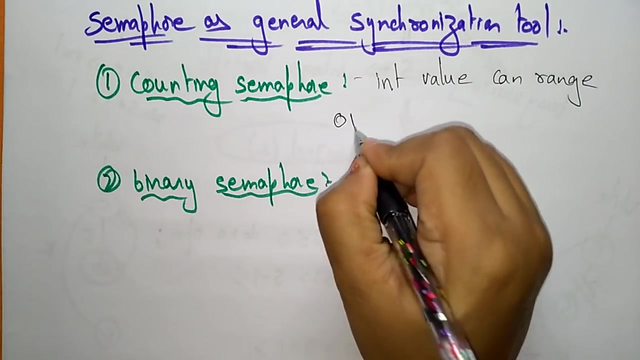 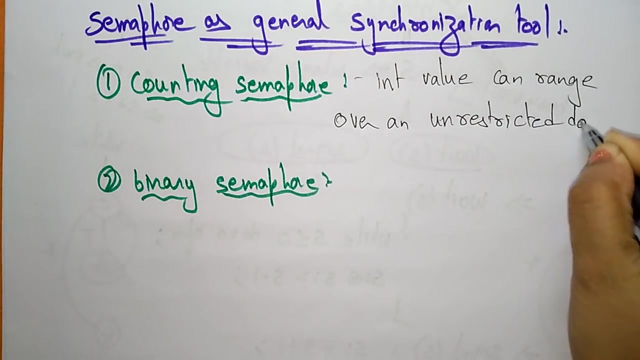 How we call this other general 2.. Here we are using the two concepts. One is a counting semaphores and another is binary semaphores. Counting semaphores means whatever the integer value we are taking, the integer value can range over an unrestricted domain, So that you call it as a counting semaphores. 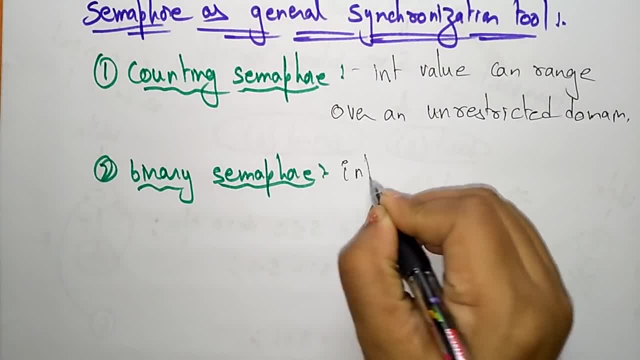 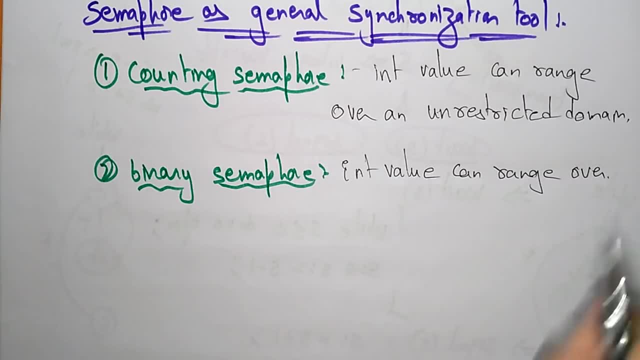 Then what about the binary semaphores? Binary semaphores means integer value can range over between only two values, that is, a 0 and a 1.. Which can be simpler to implement. So, rather than going for the unrestricted domain, if 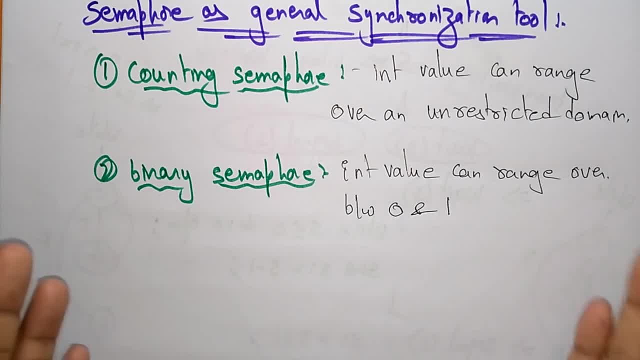 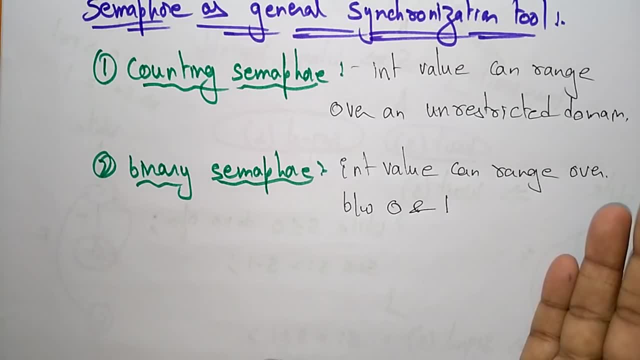 you are taking the more range of values. it is better to take only two range values: 0 and 1.. So that is the concept of binary semaphores. Binary means only it is using the two values 0 and 1. Whereas the counting semaphores means it can use the integer value that can range. 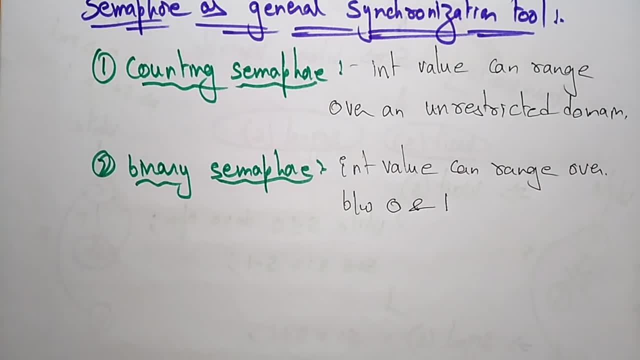 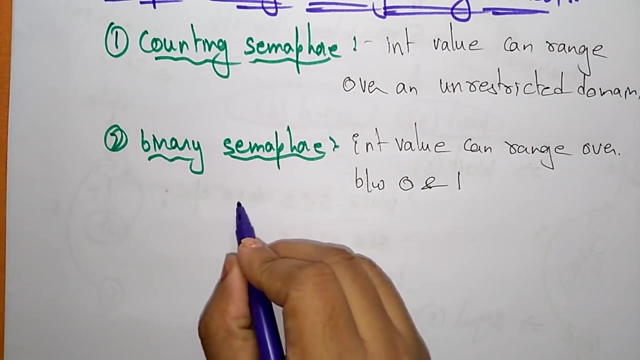 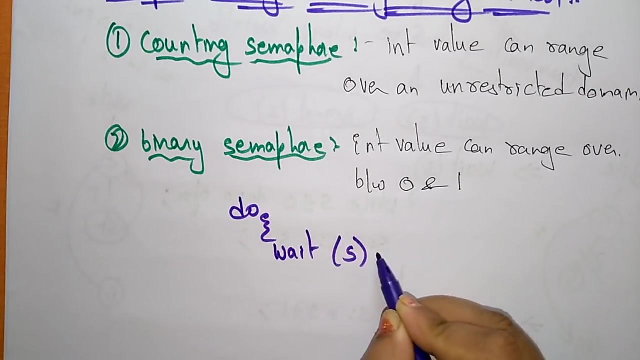 over an unrestricted domain. Okay, So this semaphores will use the two values 0 and 1.. It mainly provides the mutual exclusion concept. First. it follows the mutual exclusion concept. So let me write that semaphores code here. Do I am writing wait? semaphores value. 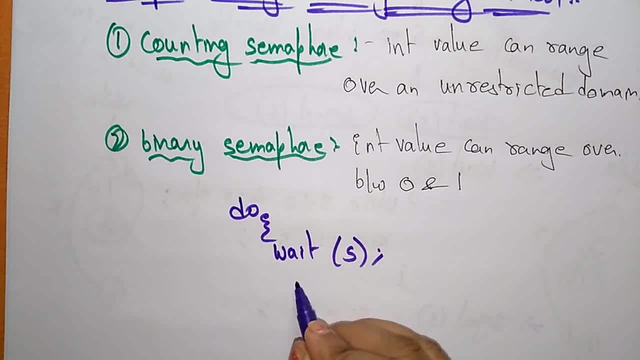 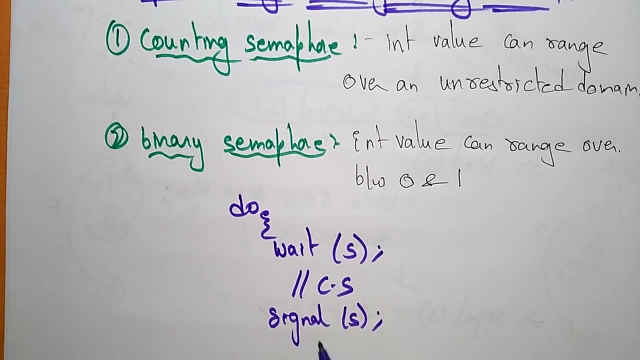 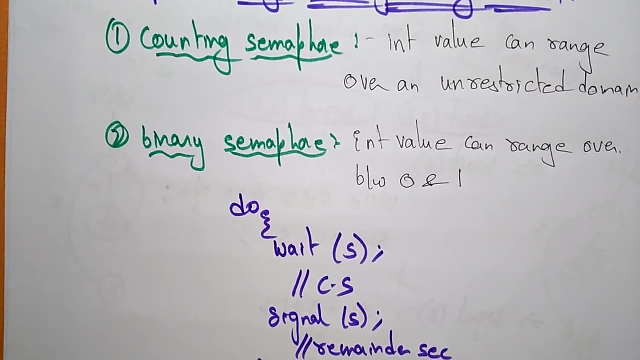 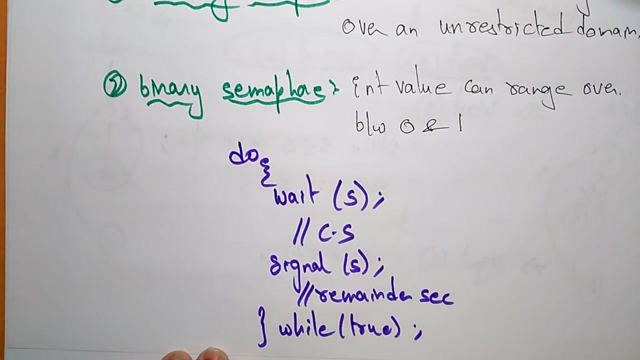 Next, critical section: Signal S, Reminder section, while condition. so this everything is about the critical section. the main thing here is we have to execute the program. which are using the resource, same resources that should be entered into critical section. so whatever the concepts here we are explaining is completely about process. 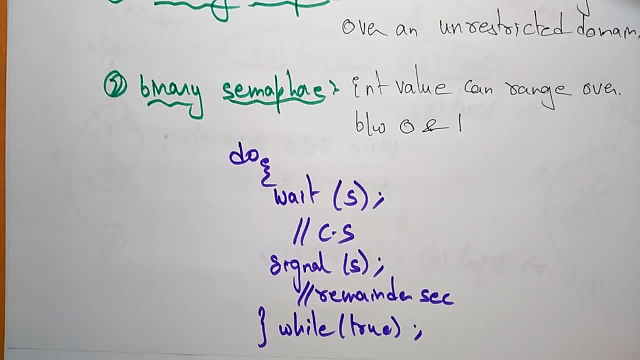 synchronization. our main aim is: we have to make the process synchronization. we have to make the program as a consistent state. you have to make the program, as it execute the program in consistent state, in a consistent state. so to maintain that process in synchronization we are using this. 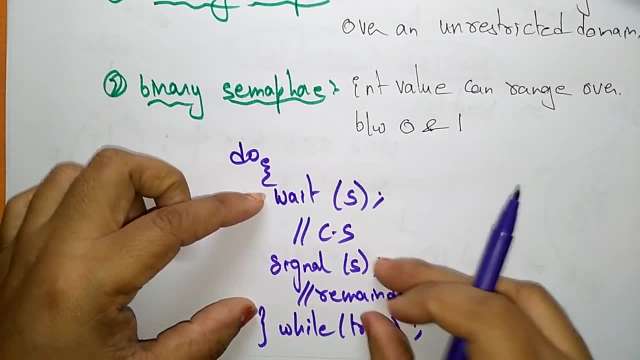 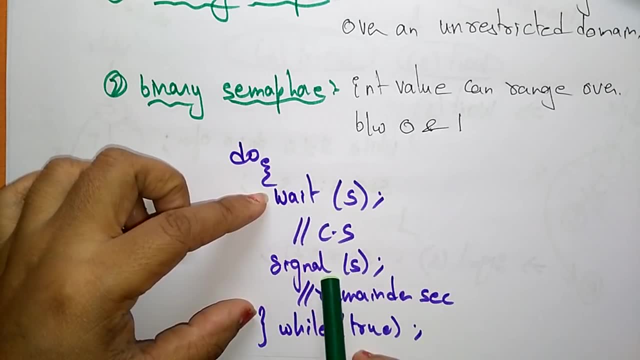 some of us value here. so here in some of us we are using to atomic variable concept. that is a weight, atomic operations, weight and weight. so this is the weight and weight of the process and signal. So in the previous mutual exclusion or in the critical section problem I just 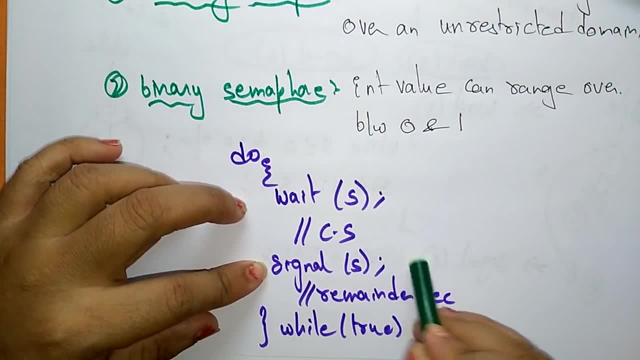 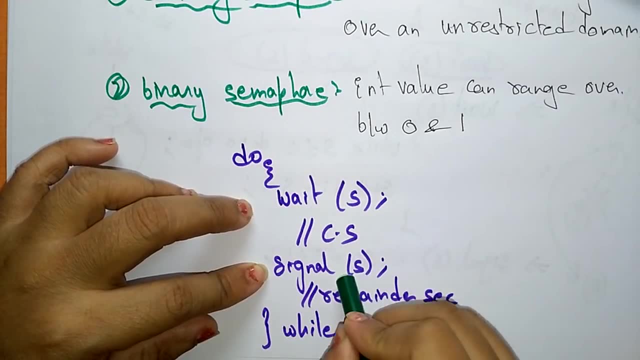 given that entry section, critical section, exit section, reminder section, But instead of entry section and exit section I am using the two atomic operations, weight and signal. Why I am using this weight and signal instead of entry and exit section? Let me explain. 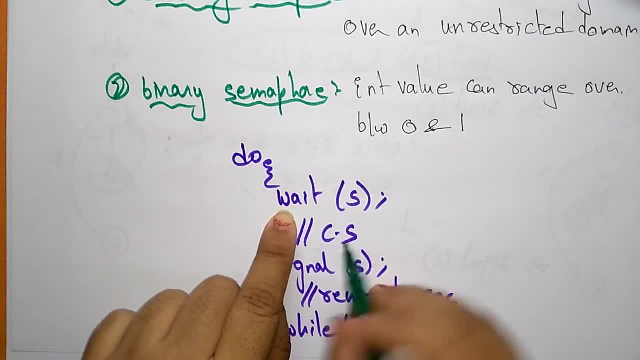 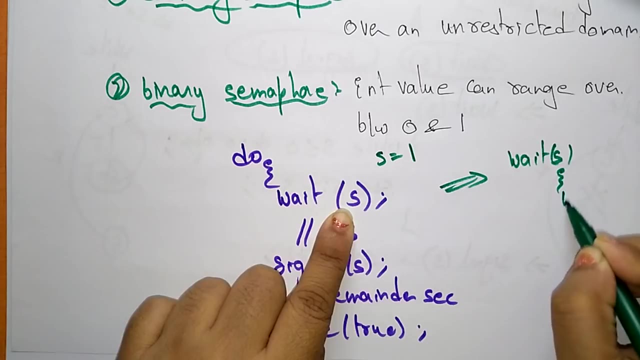 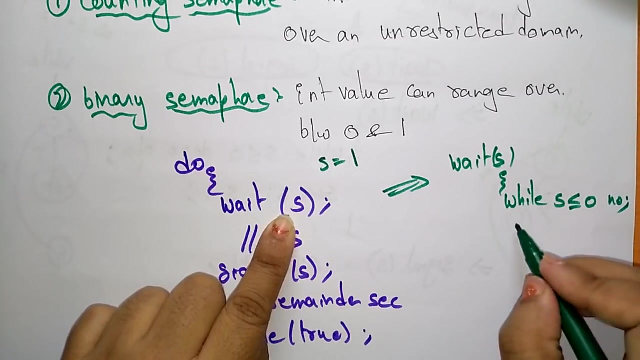 that. So here I am saying that weight s starting, the s variable, that is, the sum of s variable, should be initialized with 1.. So whenever the weight s, is there that weight program, what is that? Weight s, while s less than or equal to 0, no operation, Okay, And 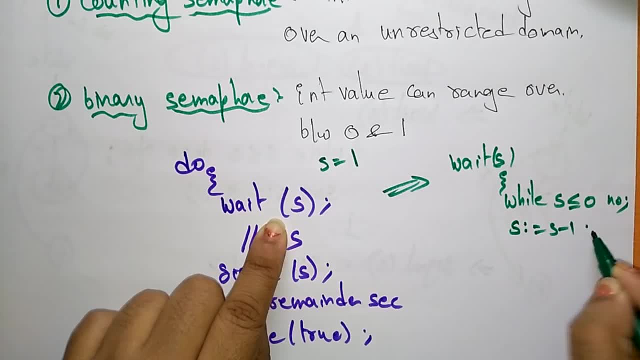 you have to decrement the s value, Exit the while loop. So whenever I call the weight s first, it takes the weight 1.. It takes the weight 1.. So it is checking: is 1 less than or equal to 0, 1 less than? 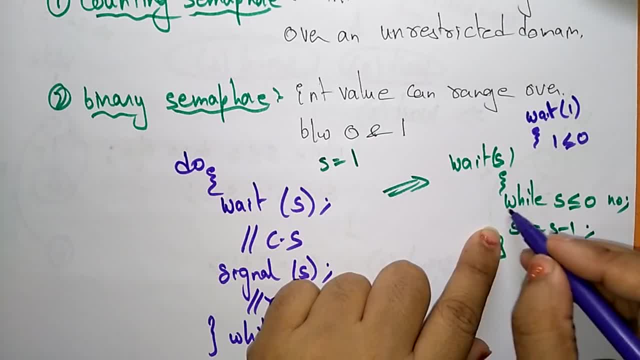 or equal to 0.. No, it is not 0.. So it exits from the while loop and decrements the s value. s minus 1 means 1 minus 1, 0.. Now here s becomes 1 minus 1, 0.. So here s becomes 1 minus 1, 0.. So here s becomes. 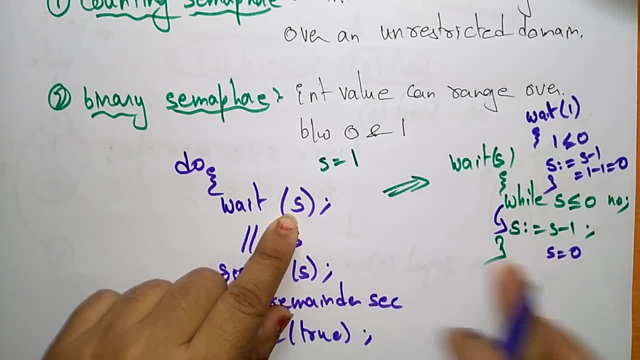 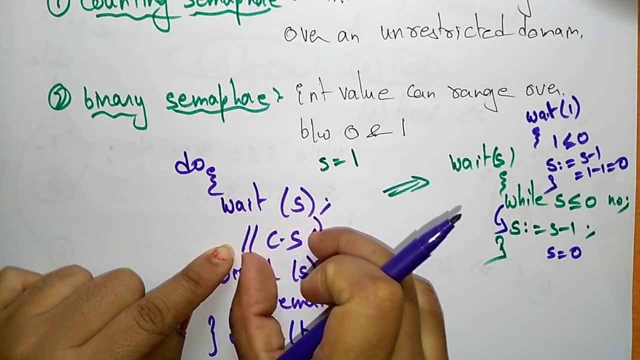 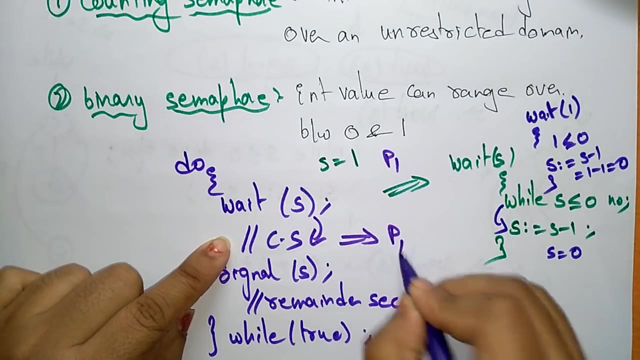 0. So whenever the s becomes 0,, then the processor will enter into critical section. So until that s will 1, the processor will enter into critical section and execute the program. Okay, That process. P1 enter into critical section Here. P1 enter into critical. 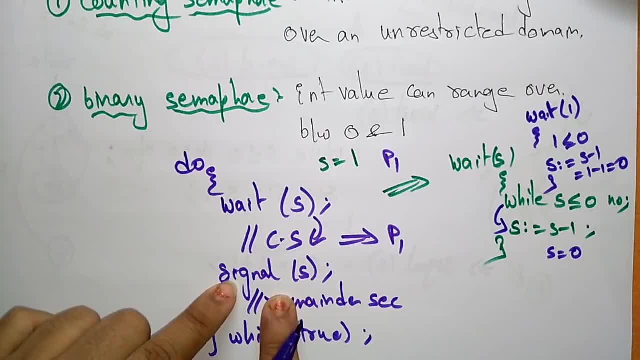 section and executing the program. Okay, After that I am calling signal s. Signal s means just: it increments the s value. S is equal to s, plus 1 means 0.. Previously s is 0.. So it increments the s value 0 plus. 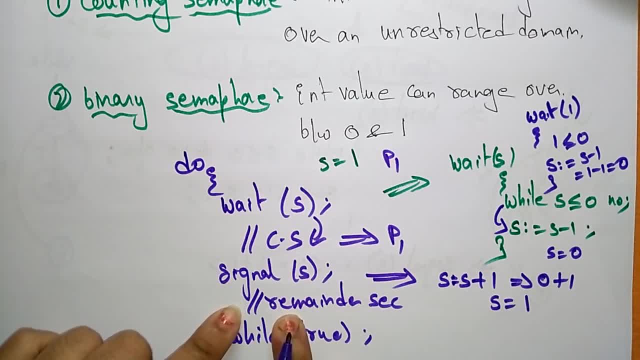 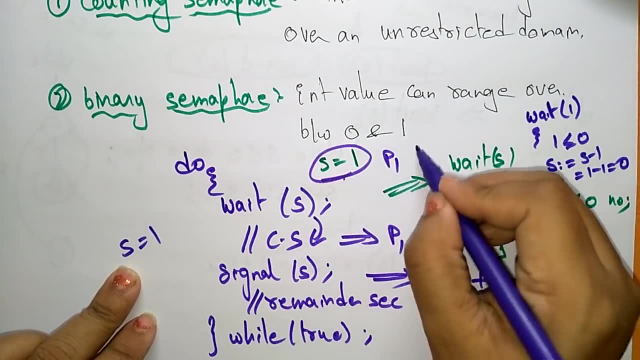 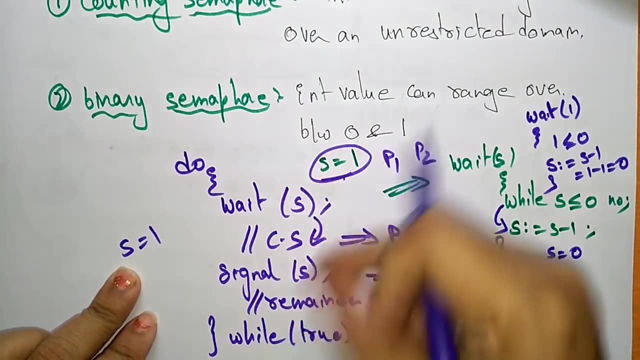 1.. Now s becomes 1.. So whenever that is s is equal to 1 means it is coming to the starting position. Next P2 process will enter into critical section. So the P2 is waiting until the s becomes 1.. So that is why we have used the weight and signal operation.